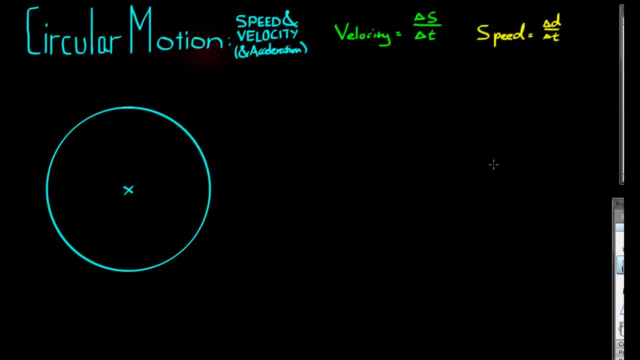 to be changing. But first of all let's look at the relationship between the speed and the period. Say, I have a ball rolling around in a circle of radius 10 meters And the ball is rolling around once every 30 seconds. So the period equals 30 seconds And the speed. 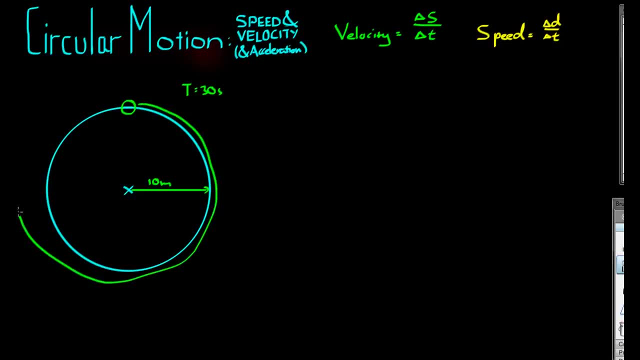 is 30 seconds. That's how long it takes for this ball to roll all the way around this circle and return to the start. Let's figure out if we want to find the speed at which this ball is rolling, which is given by v. 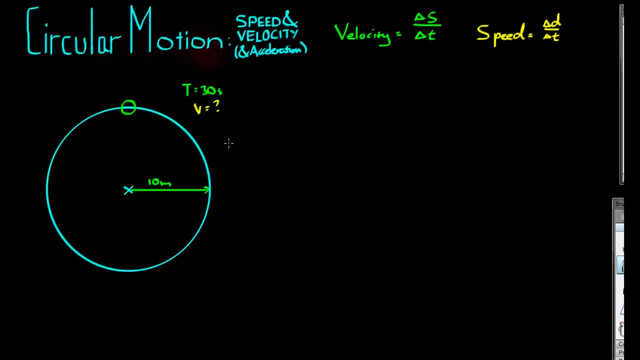 Let's figure out the total distance this ball has to roll. So we know the circumference of a circle is equal to 2 pi r, And in this case that's 2 times 10 multiplied by the pi or 20 pi, And that is the circumference of this circle, or delta d, the distance, the 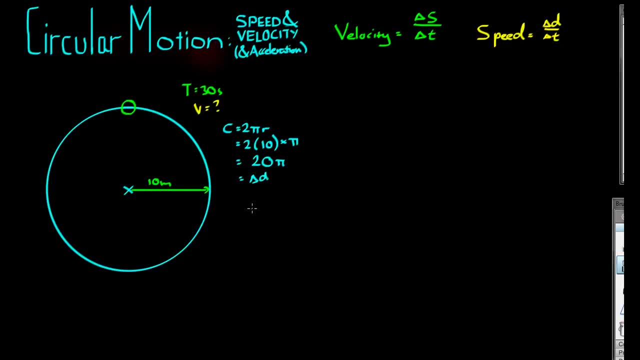 ball has to roll. So we say that's delta d And we know delta t. the time it takes to complete that distance is 30 seconds, So delta t equals 30. And under this formula here, speed, which we'll give by a yellow v, speed and velocity are both given by v. 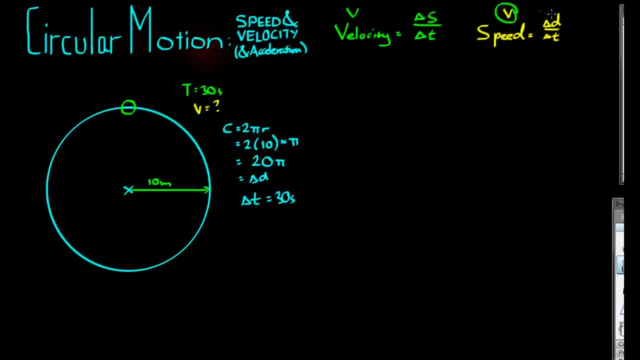 So I'm going to color coordinate here and say: if it's a v for speed, it's a v for speed, it's yellow, And if it's a v for velocity it's green. So we can say: speed v is equal. 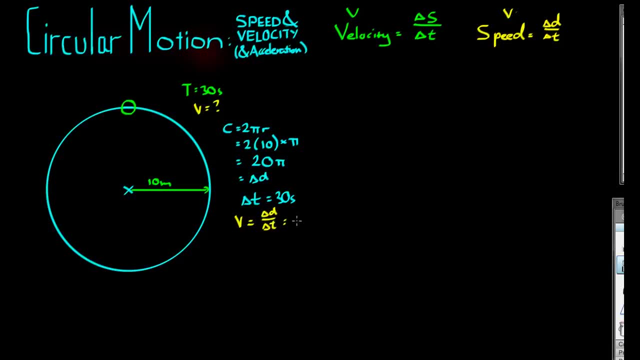 to delta d on delta t, And that's 20 pi on 30 seconds. That's also in units, that's, since it's in meters, it's 20 pi meters. So 20 pi meters on 30 seconds, that's 2 pi. 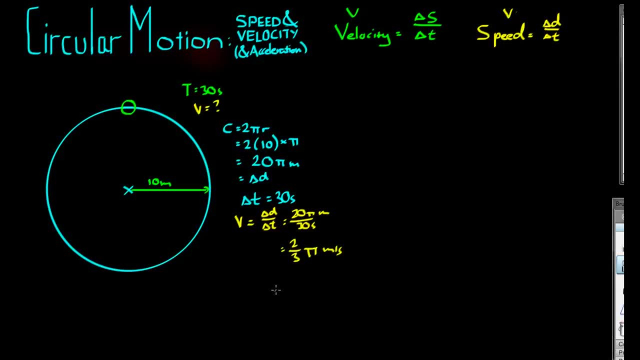 on 3 pi meters per second or round about 2.09 meters per second. So for a ball to roll around the circumference of a circle with radius 10 meters in 30 seconds, all the way it has to travel at 2.09 meters per second. We just solved for a very specific example. 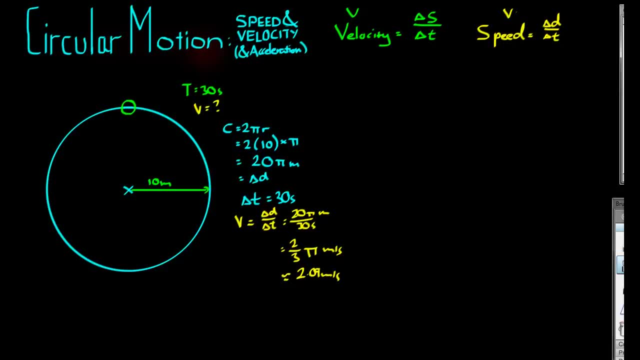 Let's solve it more generally now. Let's solve it more generally now. Say we have the speed is equal to delta d on delta t. We know that delta t is equal to the period which is given by big T And delta d is equal to 2 pi r. So delta d on 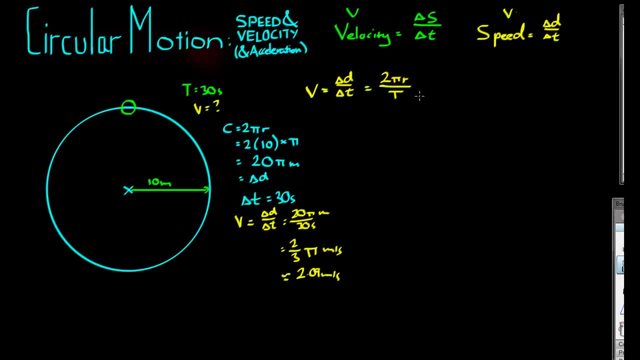 delta t becomes 2 pi r on the period. This is the general formula that relates the speed to the period, And when we use circular motion formulae, we can basically choose whether we want to work in relationship in relation to the speed or the period in order to solve for forces. 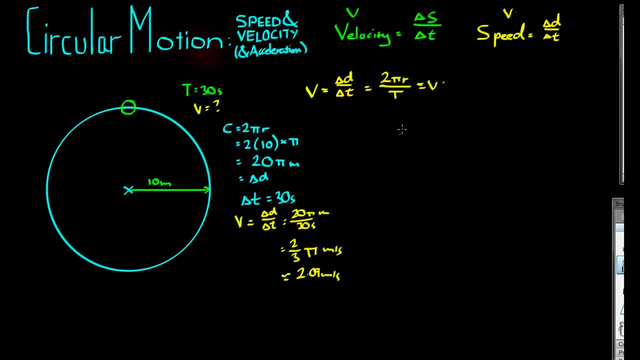 and acceleration. So this formula here, not only did we use it here to find the velocity from the period, but we can even rearrange it to say 2 pi r on v equals the period. Let's see if we can see if that works. 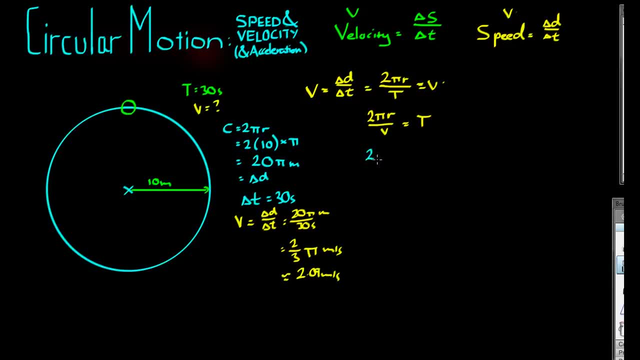 We had, v was equal to 2 on 3 pi. So 2 pi r in this case was 10, over the period, 2 on 3 pi is equal to divide everything by 2, divide the top and the bottom by pi. So we 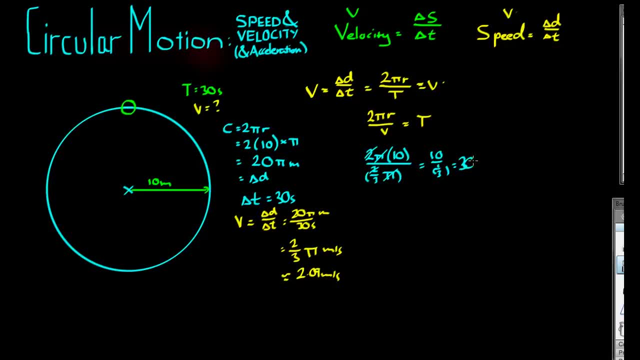 have 10 on 1 on 3, which equals 30 seconds. So it's very easy to exchange back and forth between the period and the velocity- Oh sorry, the period and the speed and the speed. I was looking ahead. Now let's discuss. 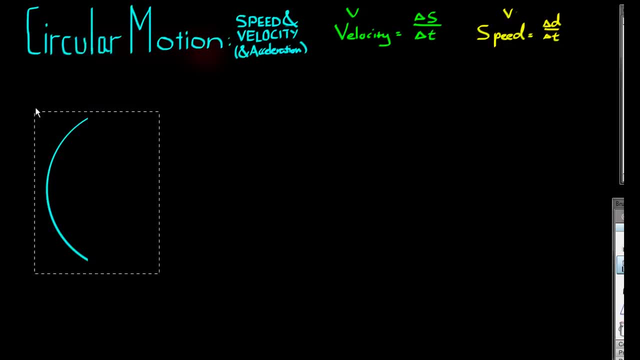 velocity. So I'll delete this, draw a new circle and title it Velocity. Velocity and velocity And constantspeed. Let's pretend this is a ferrous wheel which has carriages moving around and the wheel is turning at a constant rate. Therefore, everyone should be moving on the edges at a constant. 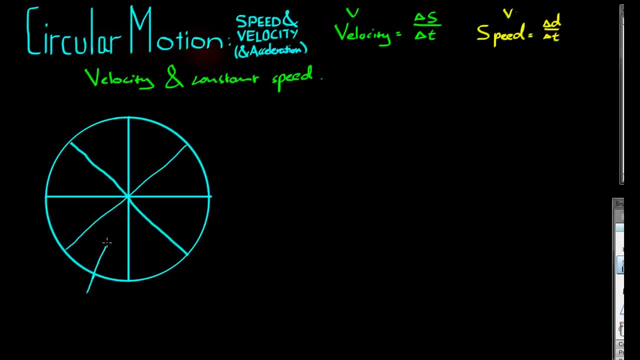 speed. However, as I said at the start, speed is a scalar. It has no direction, But once I've. But velocity does have direction and there's a very big difference between someone moving with a velocity, say, one metre a second to the right and a velocity of one metre a second directly down, and a velocity of one metre a second to the left and one metre a second up. 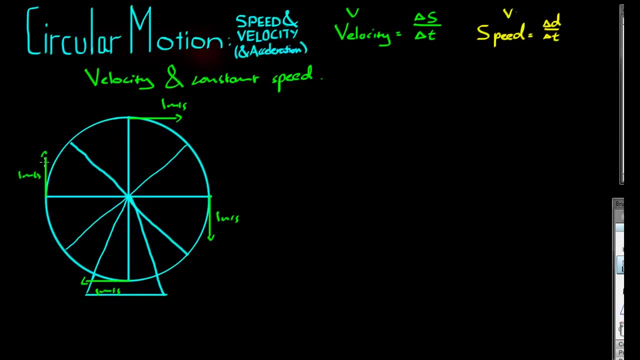 Now all these points here. we know that the carriage is moving at a constant speed, but since the direction in which it is moving is changing, we know the velocity must also be changing. And here's the key: If velocity is changing and there's also a change in time in which that's happening, it takes time for the carriage to move from here to here. 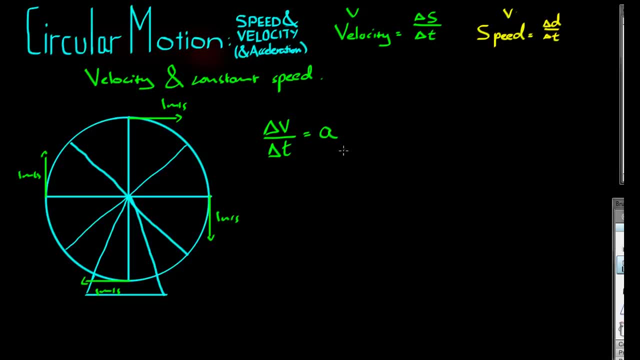 there must be some kind of change, There must be some kind of acceleration going on, And if there's an acceleration, there must also be whoops. F equals M, A. If something is accelerating, it must have a force being applied to it. 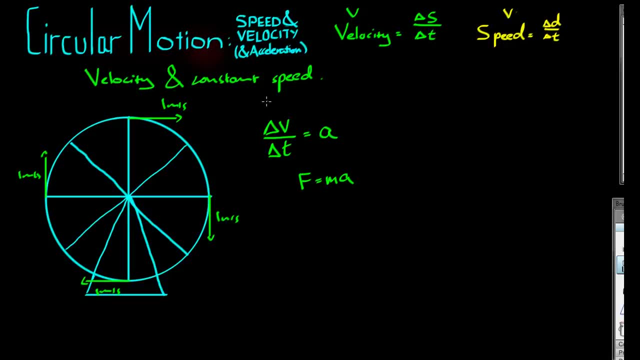 So let's look now We've discussed speed, period and velocity, Let's jump ahead and talk a little bit about acceleration. Say we have. I'll try and sketch this In the background. The best way, where is it? Expand the circle. 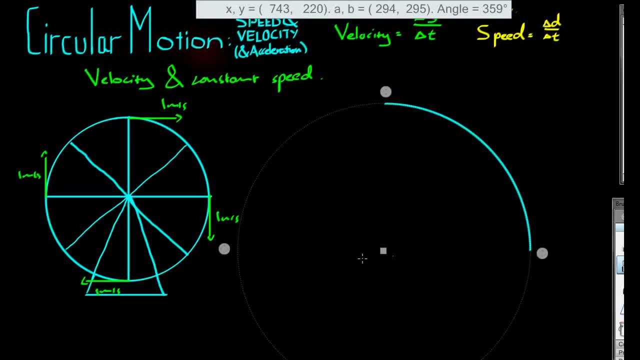 I want to draw a half circle here. That works. Say, I have a car and it starts off up here and it's trying to turn a corner. We'll say it has a mass of 1,000 kilograms And it starts off heading with this velocity. 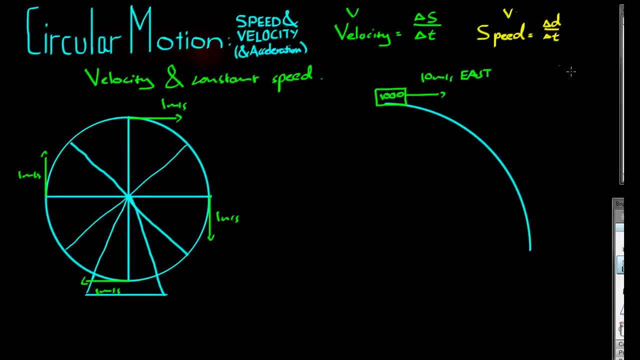 10 meters a second east. We'll draw a little compass here: North, east, south and west, And after it's finished turning it's heading 10 meters a second south And it's moving at 10 meters a second all throughout this turn. 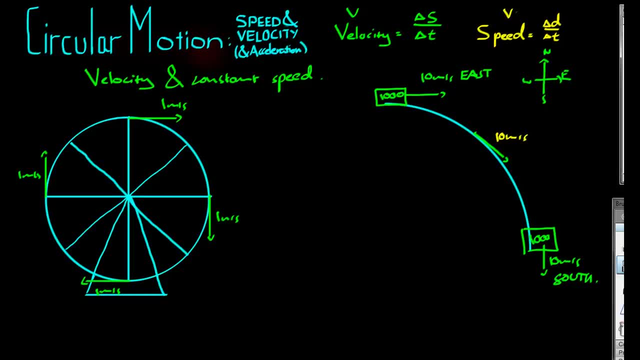 I'll mark that in as a speed. Let's figure out the acceleration for this turn. We know that acceleration is delta v on delta t And of course this delta v is a velocity, because acceleration is also a vector. So we want to figure out the change in the velocity. 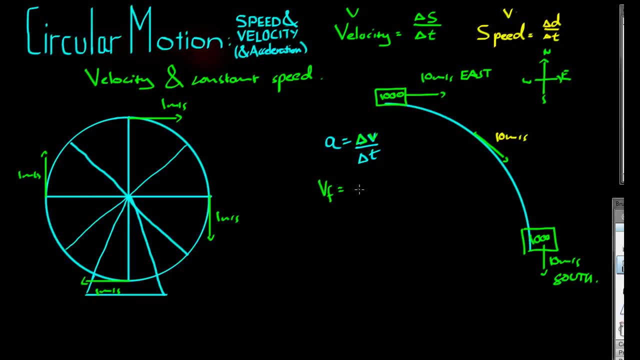 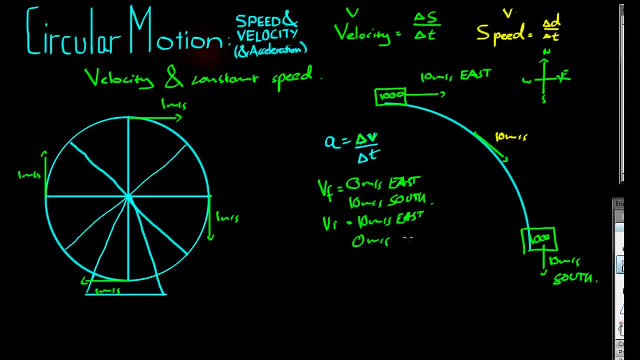 And the initial velocity is equal to 10 meters a second east and 0 meters a second south. And the initial velocity is equal to 10 meters a second east and 0 meters a second south, 0 ms south. So delta V is equal to Vf. take Vi, which comes to, let's see Vf. Vf is 0. 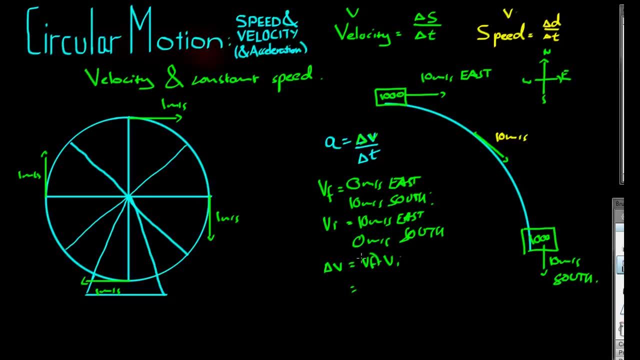 ms east, Vi is 10 ms east, So Vf take Vi is negative 10 ms in respect to the direction east. And then Vf is 10 ms south and Vi is 0 ms south, So 10 take 0 is 10 ms south. So 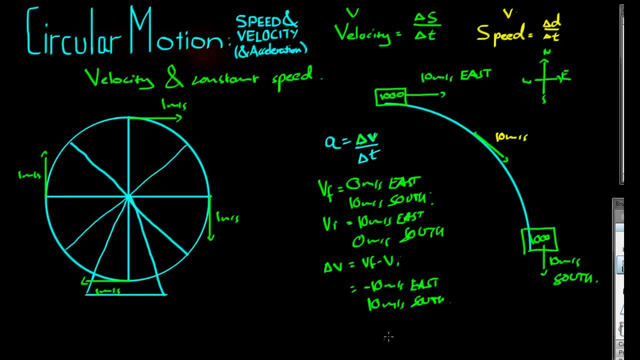 this is the change in the easterly direction and the change in the southerly direction And, of course, if we divide delta V by delta T, we'll say, in this case, delta T. it took 10 seconds to pull this turn. 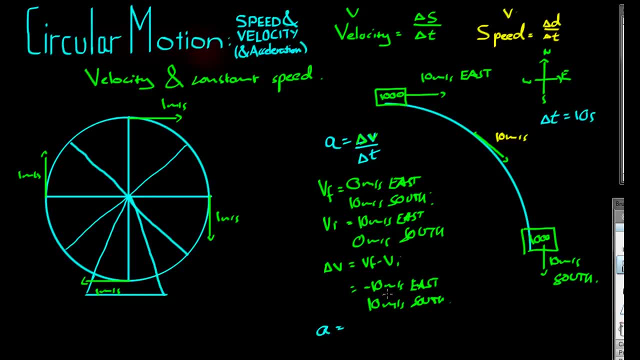 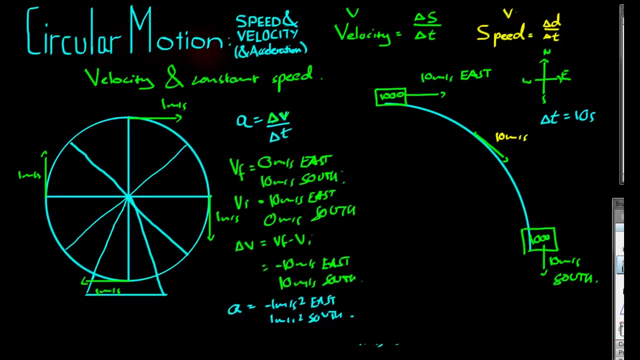 Then A. the acceleration is equal to this divided by 10, so negative 1 ms squared east and 1 ms squared south, And I'll show why this is important. I'll move this over here. We said velocity is a vector, so it has direction.